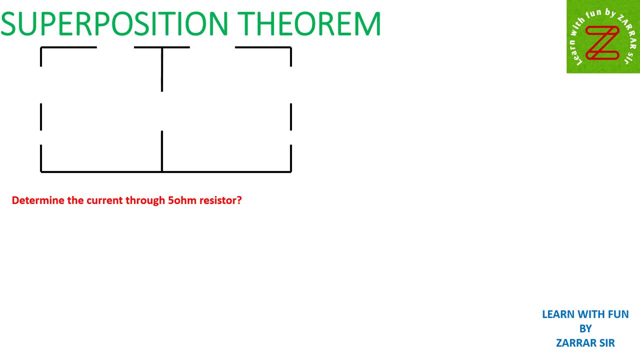 assalamu alaikum, welcome to my channel. learn with fun by zahra sir. today we're going to discuss about a very interesting topic, which is superposition theorem. so I'll make sure you understand superposition theorem with an example. so let's start with this example. I will take the resistance over here as 10 ohms. 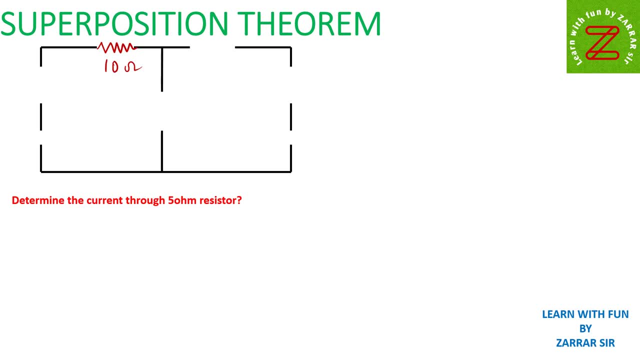 10 ohm, the resistance over here as 5 ohm and I need to calculate the current across this 5 ohm using superposition theorem and take this resistance as 10 ohm. okay, let's take some lower value resistance also, to understand it more. 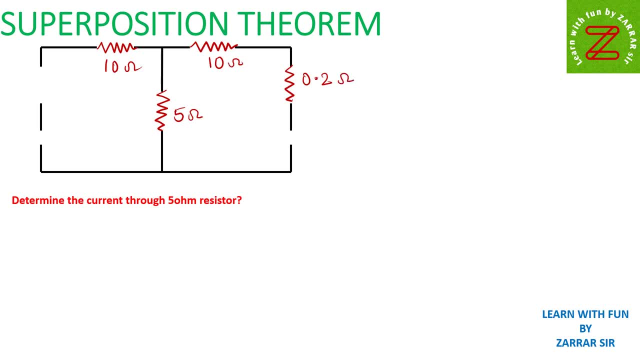 precisely, I will take it as 0.2 ohm. okay, and I'll take this resistance as 0.1 ohm. okay, I'll take this voltage as 2 volt. okay, I'll take this voltage as 2 volt. I'll take this voltage as 4 volt. now let's try to. 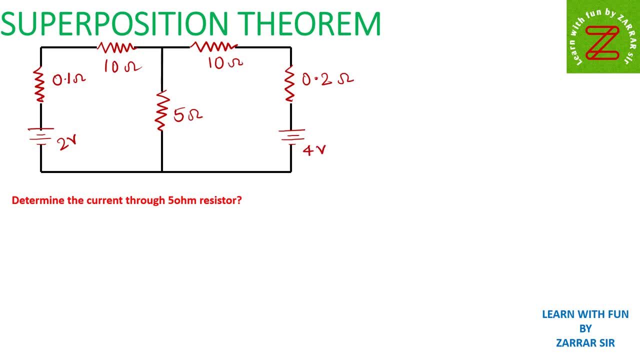 analyze this using superposition theorem. if it, if this problem needs to be solved using KVL, then it is very simple. but now let's make sure that you understand the problem first, and then we'll talk about. I will try to make sure that you understand this using superposition. 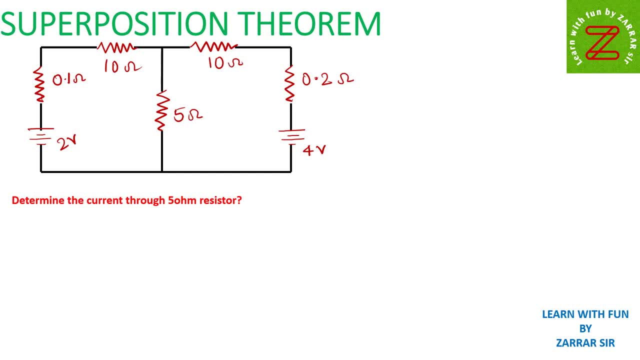 theorem. it is very easy and very interesting topic. in superposition theorem, there's one concept that you need to remember, okay, which is we have to consider one source at a time. okay, consider one source at a time, only one source, and make sure, whenever you consider one source at a time, you should. 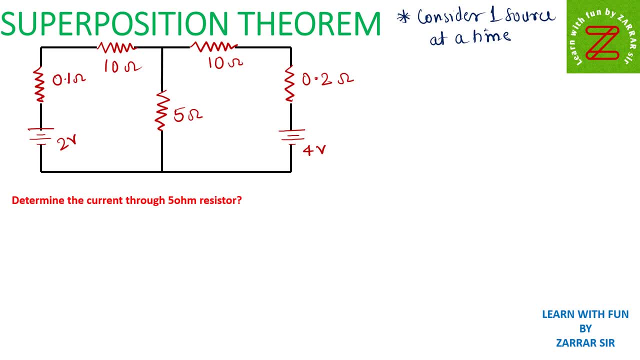 consider one source at a time, only one source, and make sure, whenever you considered one source, make other source depend on their internal resistance. like we are considering voltage source, make other sources voltage source has to be a shorted and while you are considering voltage source, and if there, 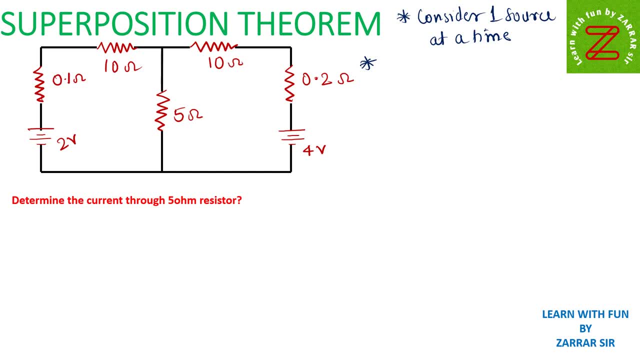 is any current source present in the circuit, make it as open, okay. so let's try to analyze this. so the first step is: I am considering 2 volt, so there is one more fulfilled and understand that the current source also. I am considering 2 volt resources, so the original voltage source is 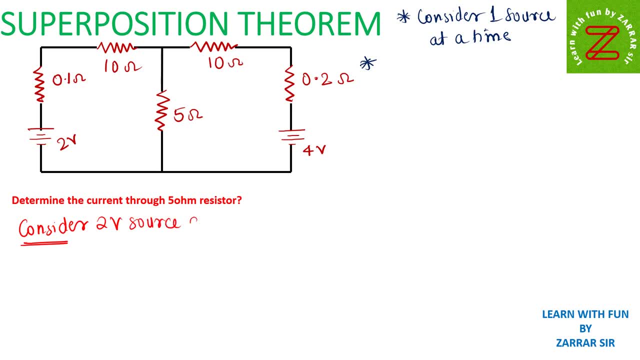 acting alone. if I consider two volt source acting alone acting alone. okay, so now I am considering two voltage source, two volt source acting alone. now see, you have to short this voltage source. I will short this voltage source, which is four volt short this voltage source, and I will apply KVL in this two loop. this is: 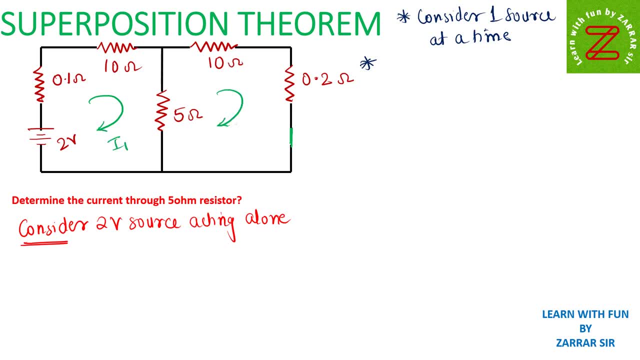 first loop and this is second loop. I'll name it as I1 and I'll name it as I2. now, if you apply KVL- you know the shortcut of KVL right, which you have already learned- you have to add all the resistance in the first loop, okay, you? 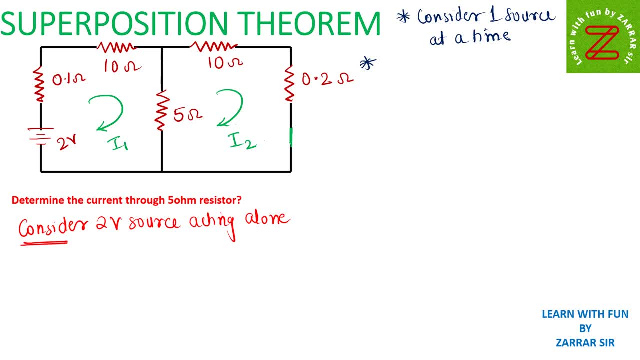 have already learned the shortcut. what to do? you have to add all the resistance. I am applying KVL in loop 1, applying KVL in loop 1. if I apply KVL in loop 1, what will happen? 10 plus 5 plus 0.1 is 15.1. so 15.1 I1 right, 15.1 I1 minus 5 I2- okay, this. 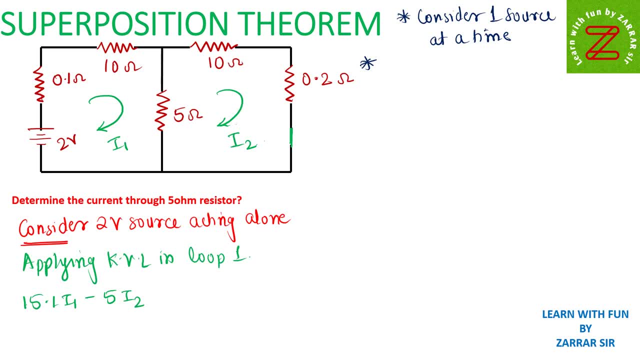 resistance is in second loop also, so minus 5 I2 is equal to 2 volt. this is my equation number one. okay, this is my equation number one. now let's take equation number two. if I apply KVL in loop 2, what will happen? bedroom, I'm applying KVL in loop 2, applying KVL in loop 2 and if I apply? 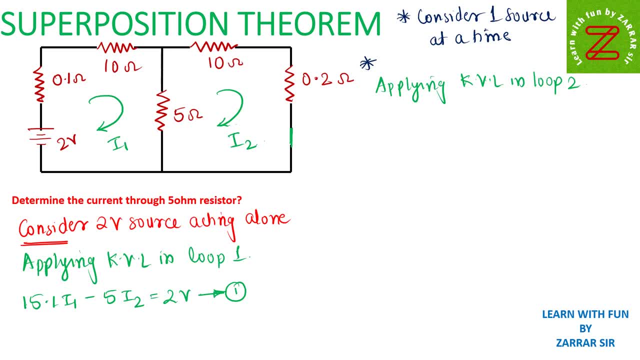 KVL in loop. to what will happen. just add all the resistance of the loop to 10 plus 5 plus 1, 2 becomes 15 point 2. so I'll write: plus 15 point 2, I2. and this 5-ohm resistance is in loop 1, so minus 5, I1. you know the shortcut. I've 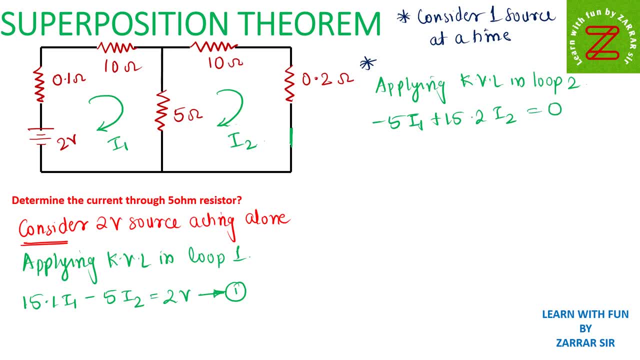 already taught you in kvl video, is equal to zero. so now you have two equation and two unknown and if you solve two equation and two unknown using simultaneous equation, you will get the value of i1 and i2. i'll directly write the value of i1 and i2. you'll get i1 over here as i1 over. 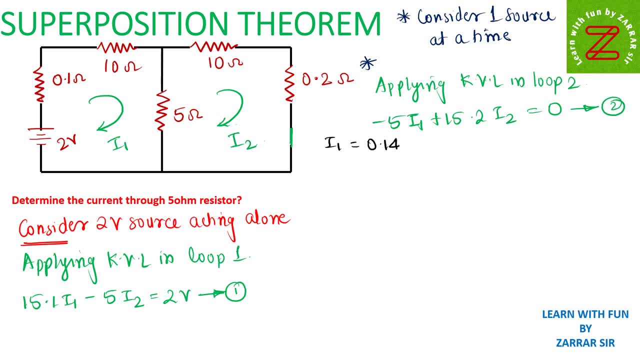 here as 0.0141 ampere and i2 over here as 0.0028 ampere. 0.028 ampere. okay, so this is i2. now, if you look properly, the current flowing through 5 ohm resistor is this: is this current, which is i1 minus i2, so i'll name it as i dash: equal to i1 minus i2. 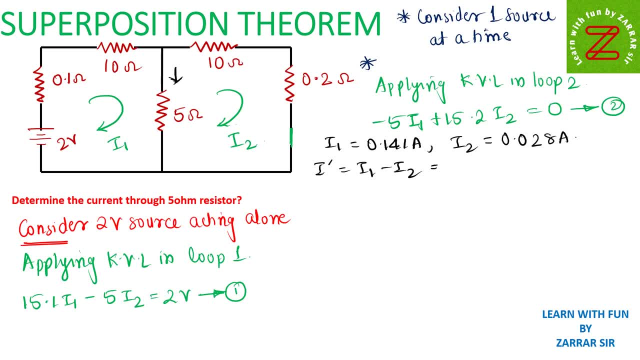 and if you subtract i1 minus i2, you will get voltage as 0.113 ampere. this is your i dash, the first current right. when you considered two volt source acting alone, this two volt source was acting alone. now we'll consider the source which we have not used. 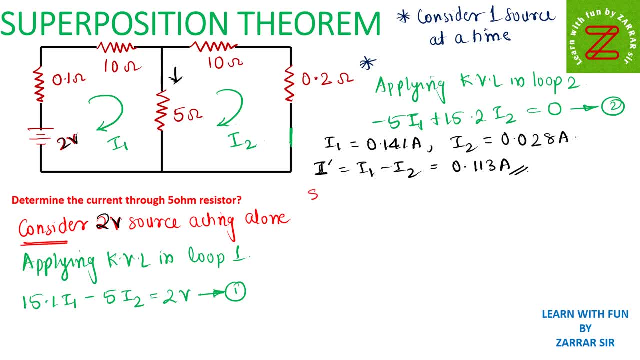 till now. so this is the next step. i named it as step two. okay, let's name this as step one. so step two is considering four volt source acting alone. okay, now, consider four volt source acting alone. now i'll erase this two volt, okay, and i'll make short over here and now. 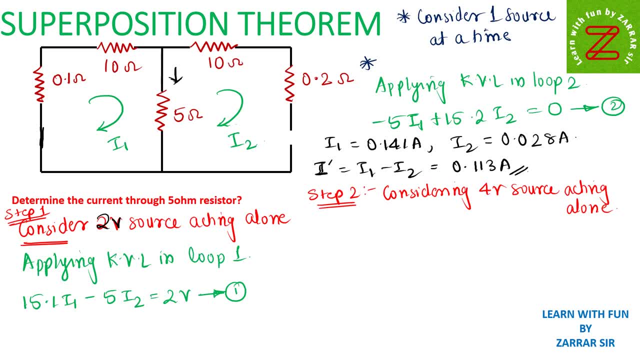 i'll erase this path and i'll draw four volt source. okay, let's draw four volt source. so this was my four volt source, and now i'll apply again kvl. so if i apply kvl in loop one, if we apply kvl in loop one, what will be the equation again ten? see, this is ten plus five plus point one becomes. 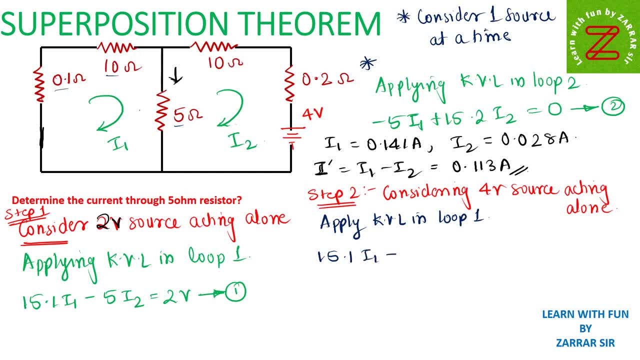 15.1 I 1 minus 5 I 2, since 5 ohm is, in another loop, equal to 0. this is the equation number 3. okay, now if I apply KVL in loop to apply KVL in loop to: if I 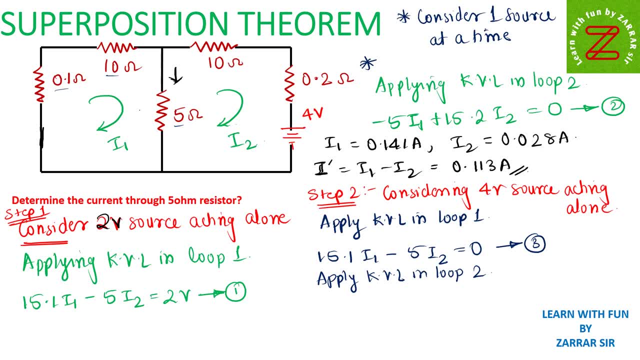 apply KVL in loop to now see what happened: 10 plus 5 is 15. 15 plus point 2, 15 point 2. this resistance is in this loop, so I'll write: minus 5, I 1 plus 15 point 2, I 2, equal to now. we have a voltage over here which is positive. 1st. 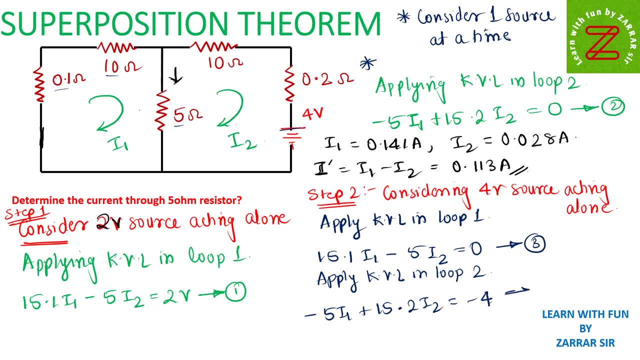 so I'll write minus 4 and this is my equation number 4. now, if you solve this equation number 3 and 4 simultaneously, you will get the value of I 1 and I 2, so I will get I 1 equal to. I will get I 1 value as. 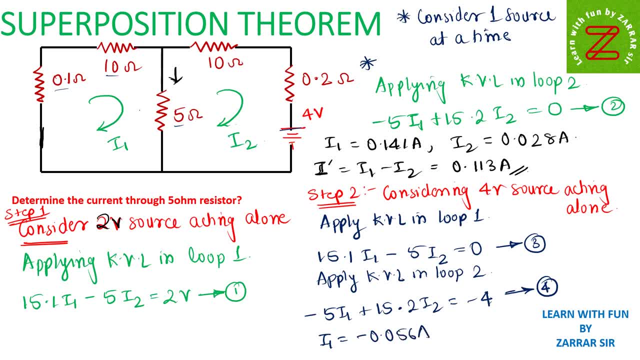 minus 0.056 ampere. okay, and you will get I 2 s I 2, you will get s minus point one six nine ampere. okay, what is your current flowing through five ohm resistor? it is I 1 minus I 2. again, I'll name it as I double dash and your I double dash will. 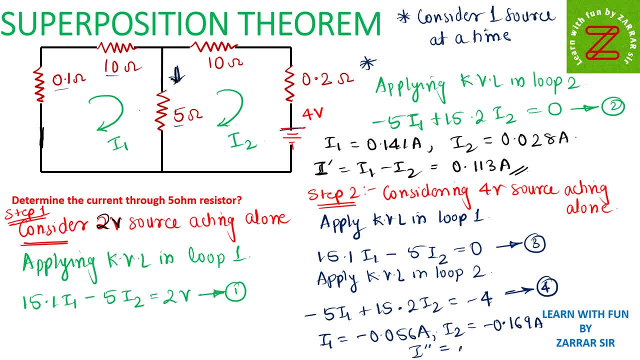 be I 1 minus I 2, and if you subtract this you will get again zero point, one, one, three ampere. okay, see, it looks both. the value looks same, but it is not always same in this problem. I got this value as same, so this was I dash in. 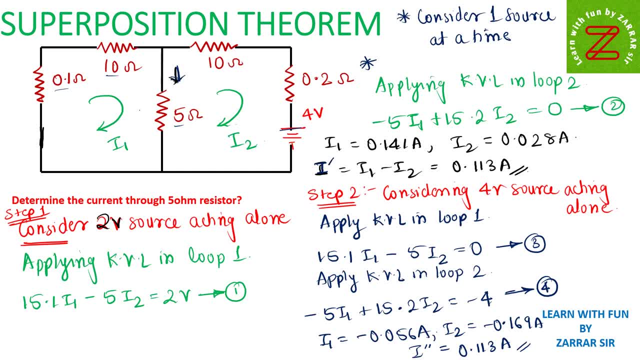 first loop in. I mean to say when I consider two volt source. this is I double dash when I get I when I consider four volt source acting alone. now, according to superposition theorem. I'm very sorry, I have not. you left the space. I am using this space over here. so when you use superposition, 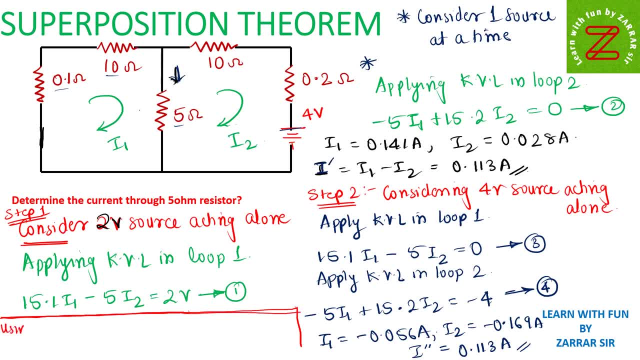 theorem. so using superposition theorem, if you use superposition theorem, using superposition theorem, you'll write: I dash plus I double dash, and which is: if you add 0.013 plus 0.0, 1, 1, 3, 1, 1, 3, 1, 1, 3, you'll get 0.25 to 6 Ampere. so this is your final answer using 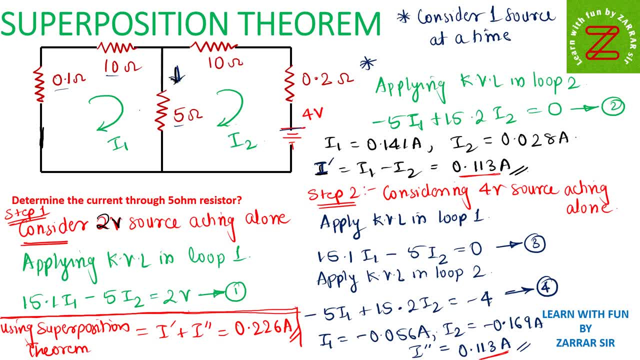 superposition theorem. this was first. I mean, this is the way to calculate superposition theorem. two voltage sources are given. now let's consider another problem with one voltage source and one current sound. okay, hope you understand this within 10 minutes: how to apply superposition theorem if you have to wallet this world, if you don't want to apply superposition. 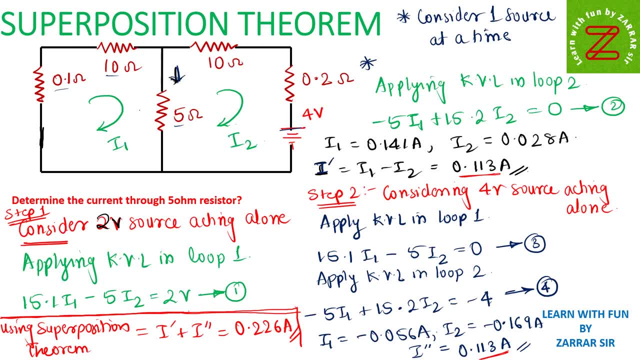 theorem if we went when we applied to the equation. when you apply superposition, ask to do supervision. you can directly solve this using KVL, which you have already learned. now let's take another problem with one voltage source and one current source. okay, so I'll move. 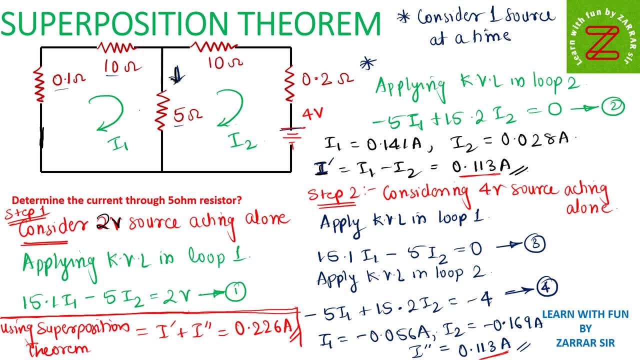 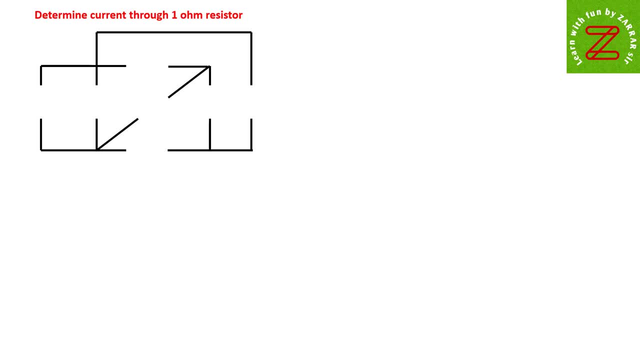 to the another problem with one voltage source and one current source. this is the problem with one voltage source and one current source. now I'll make a one voltage source and one current source over here and let's see we can analyze this problem or not. so I'll make this problem of 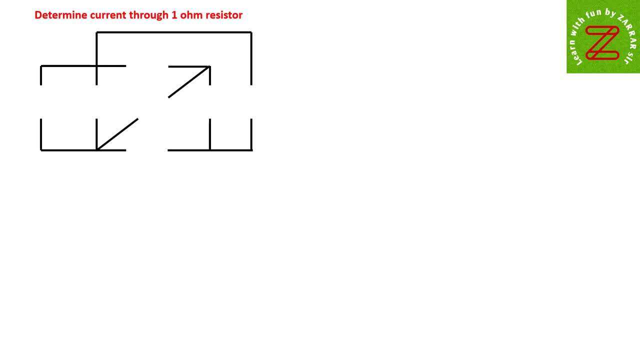 one voltage source and one current source so that we can understand this problem and we can apply the logic properly. so I'll be using current source over here and I'll name this current source, as I'll take the current source value as 1 ampere. okay, let's take this. 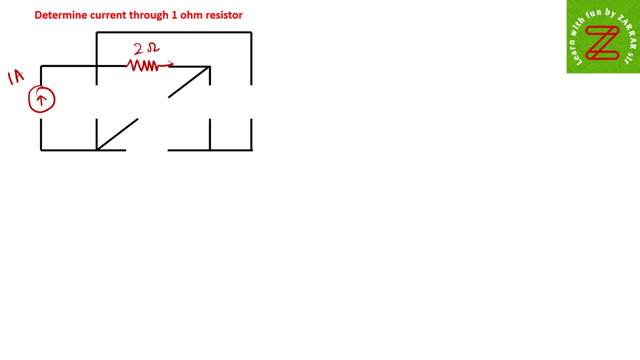 resistance, as we'll take a very small resistance, 2 ohm. okay, let's assume there is a voltage source over here which is 1 volt. I purposely taking the one world voltage source in between so that we can understand a complex problem also and you are able to solve the complex. 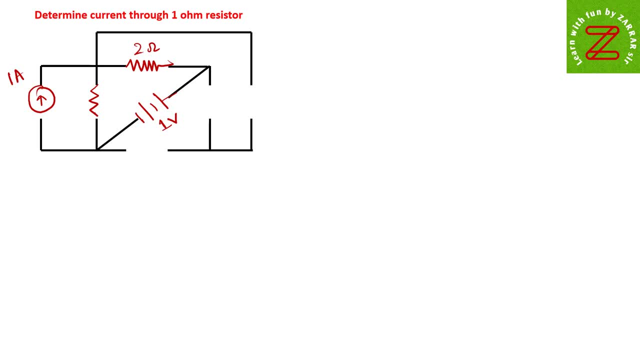 problem. also, let's take this as intense as 3 ohm. let's take one more resistance over here. I'll take it as 2 ohm. okay, let's take one more existence over here- 2 ohm- and we'll find, try to find, this value of resistance. 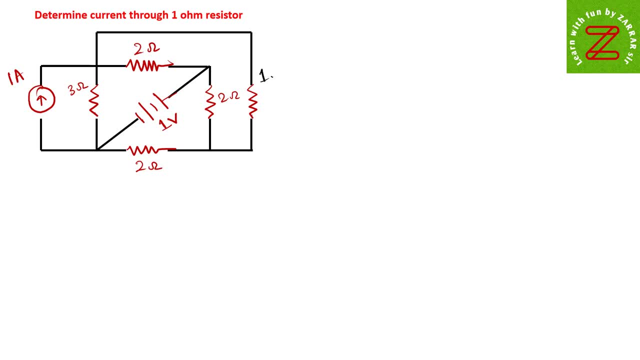 resistance, which is one ohm, which is outside the loop. okay, so this is the problem. now you can see there is one voltage source and one current source. and now how to solve such problem with one voltage source and one current source? this is a difficult, or i would say, tedious task. so now we will. 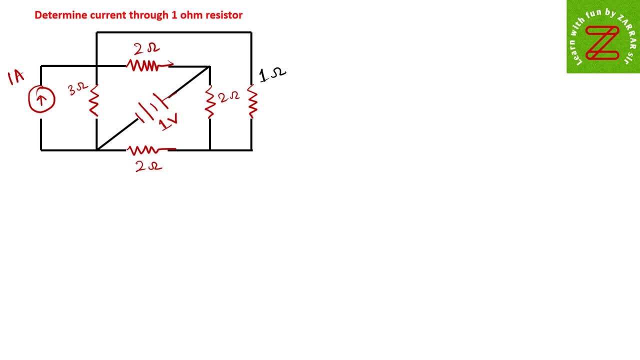 understand superposition theorem with one voltage source and one current source. now to solve this, we'll start with first step. we will consider only one source at a time, so i am considering first current source. one ampere source acting alone. okay, acting alone now, it's all your choice. 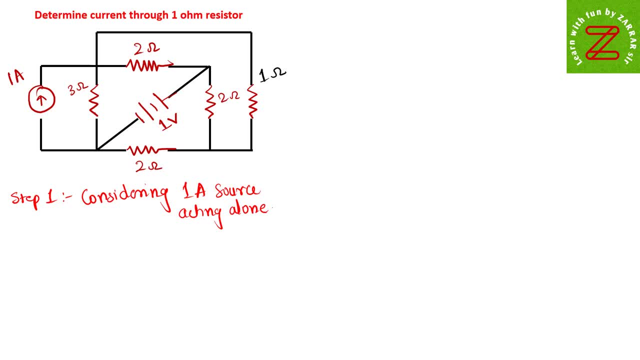 you can consider one volt also. i am considering one ampere current first. so you are aware about when you consider voltage source, you have to open current source and when you are considering current source you have to short voltage source. so i'll short this voltage source, i'll remove. 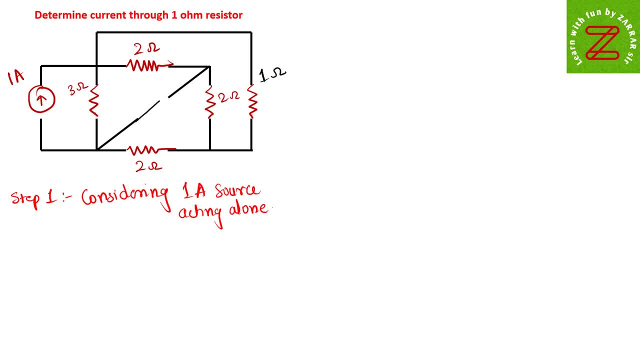 this voltage source. it was here. i will close it. i will close it and i can also perform correct love to electric current curve dürfen not done. it's not possible if you creating and I will short this terminal. okay, this is one volt source has been removed now. 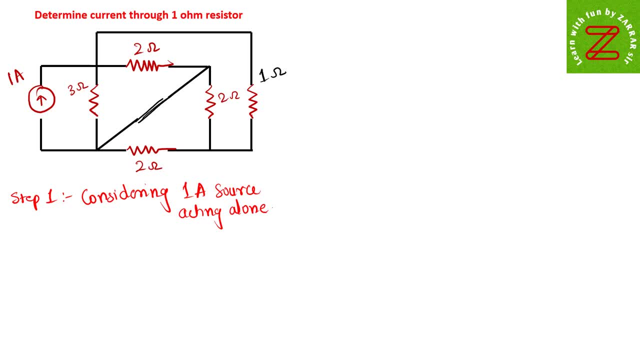 you apply KVL, which you have already studied. okay, so I will take KVL. I mean, I will apply loop current over here. I1. okay, let's take this to be as I2, I3 and I4. I2, I3 and let's take this as I4. from as you can see, the problem looks very. 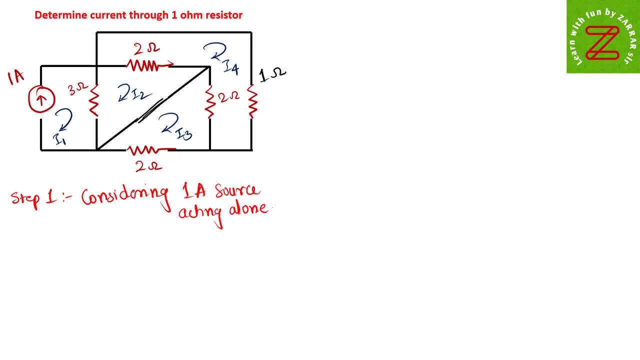 tedious because there are four current source and how we can solve four current source. I mean four current equation in an calculator. but if you look, look properly, you can directly write. this is the current I1 which is flowing in this loop and there is a directly current source given. so you must be aware about 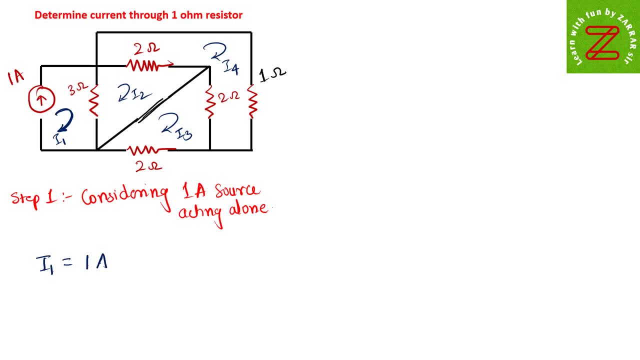 a concept that we can write: I1 is equal to I2 and I3 is equal to I3 and I4 is equal to I4 to I3 and I4 is equal to I4 and I5 is equal to I4 and I5 is equal to 1 ampere directly, Since there is 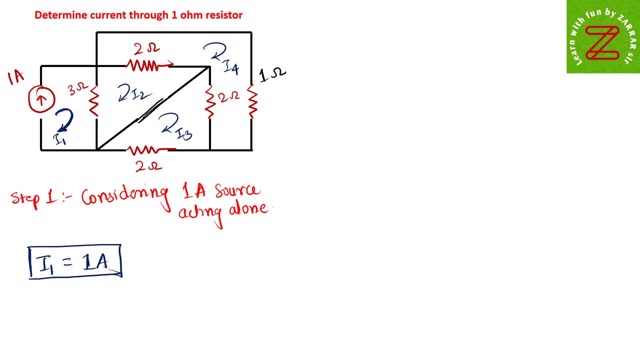 no other current in that loop. so I1 is directly what 1 ampere, which is a very simple part of the problem. Now let's try to apply KVL in loop 2.. So when I apply KVL in loop two, if you apply KVL in loop 2, you can see if you apply KVL in. 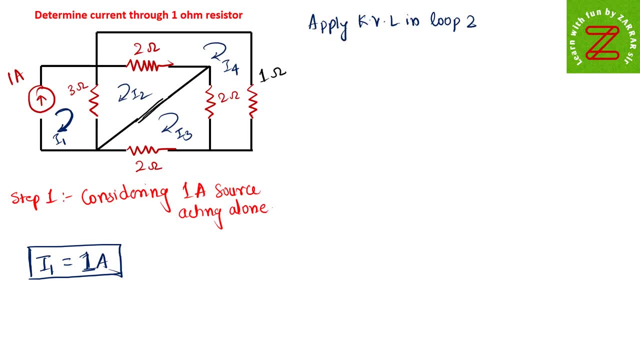 loop 2. what you are end up with you can directly write with the shortcut: 3 plus two is five. three plus two is five five, 5 I 2. minus this 2 ohm is in fourth loop, also minus 2 I, 4, equal to 0. so this is: 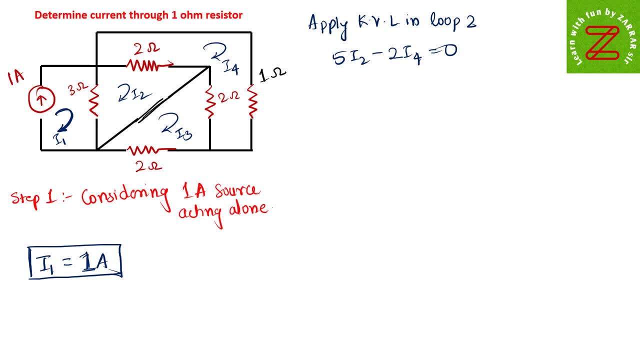 very simple equation: right minus 2 I 4 equal to 0. so which is very simple. but if the student make mistake because they forget to consider this resistance 3 ohm, see I 2 current has 2 resistance 3 plus 2, 5 I 2, 2 ohm is in fourth loop also, so I 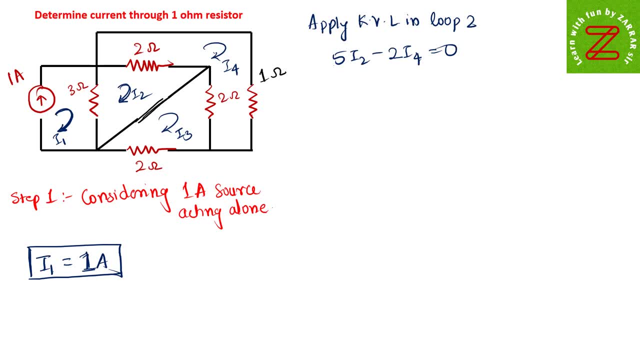 have write written minus 2 I 4, but 3 ohm is in first loop, so we need to consider that 2, so we cannot write 0. we have to consider that resistance, which is minus 3 I 1, equal to 0, and you know the value of I 1 is 1 ampere, so you can. 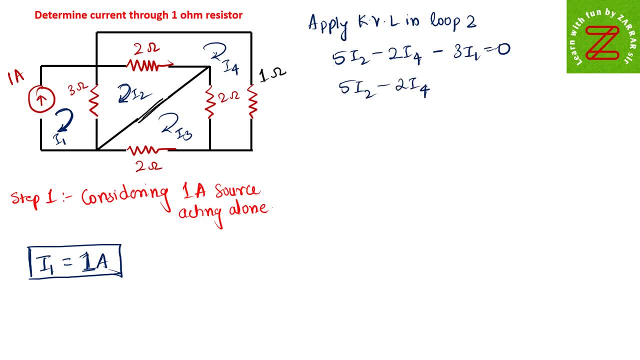 directly write 5 I 2 minus 2, I 4 minus 3 into 1 is minus 3, which will go over there and write 3, so this is the equation number 1. I'll write okay, so you hope you are understanding. I have used this two resistance as 5 I 2 minus 3, I 1 minus 2, I 4 equal to 0 and 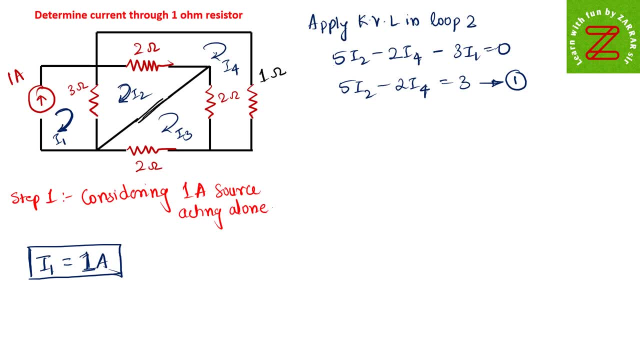 you have the value of I 1. you have substituted the value of I 1. you get this equation. now I'll apply KVL. applying KVL in loop, very sorry. applying KVL in loop 3. okay, if you apply KVL in loop 3, what you end up with 2 plus 2 is 4. 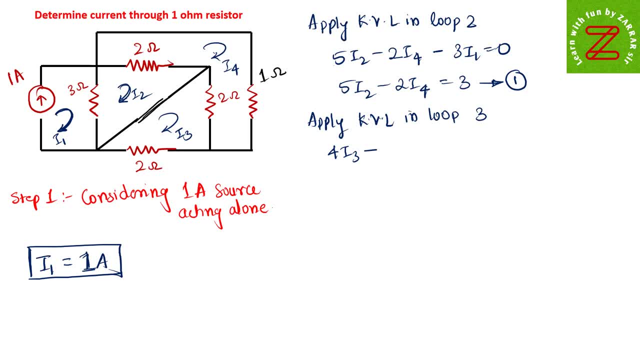 I 3, 4 I 3 minus this, 2 Ohm is in fourth loop, also minus 2 I 4, equal to 0. so this was very simple equation, okay, and now I'll apply KVL in fourth loop, also applying KVL in loop 4, and if you apply, I write this equation number 2, if you. 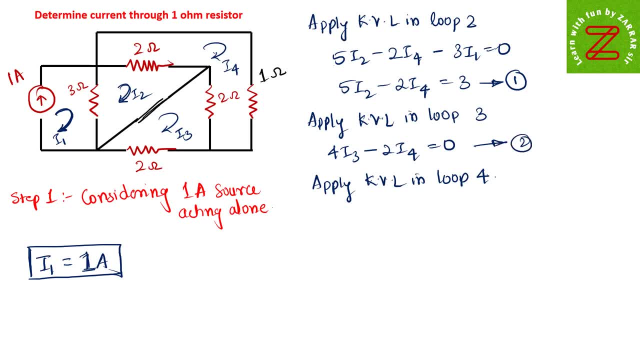 apply KVL in loop 4: 2 plus 2 plus 1 is 5 ohms, so 5 I4 minus. this 2 ohm resistor is in third loop also. so minus 2 I3, this 2 ohm resistors in second loop also minus 2 I2, equal to 0. so this is my equation number 3, as you can see. 3. 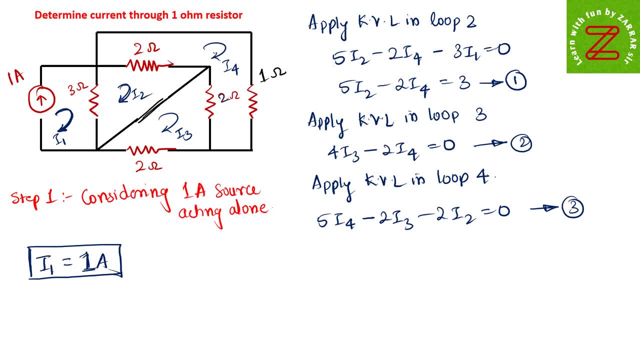 equation has 3 unknown- I2, I3 and I4, and if you solve this in calculator, you will get the value of I2, I3 and I4, as I will get the value of I2, as if you solve it into calculator, you will get my. 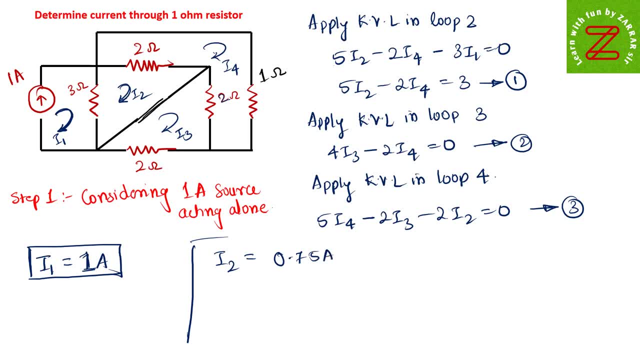 0.75 ampere of I2, which I have already solved. I3, equal to you, will get 0.1875- okay, and I4, you will get it as 0.375, 0.375 ampere and if you look carefully, we need to calculate. 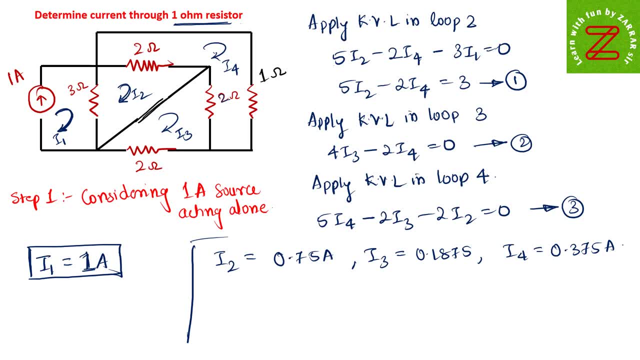 determined current through 1 ohm resistance and the current through 1 ohm resistor is this current, which is nothing but your I4, so I can directly write: my I dash is equal to I4 is equal to 0.375 ampere. so this I have get the current. 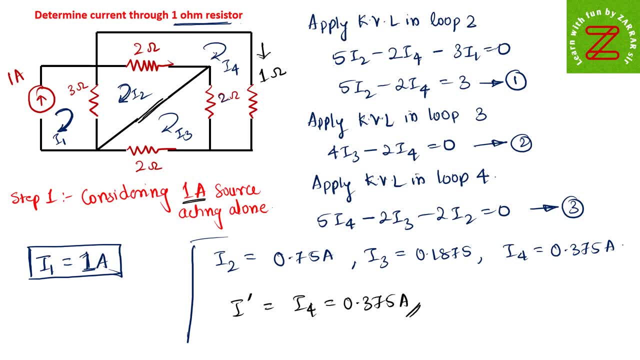 only when 1 ampere source is acting alone and we have removed the voltage source. now, in the next part, we will add this voltage source and we will try to analyze the equation. so let's add the voltage source and remove the current source and you are aware about. if I add the voltage source, I need to open the current source and the 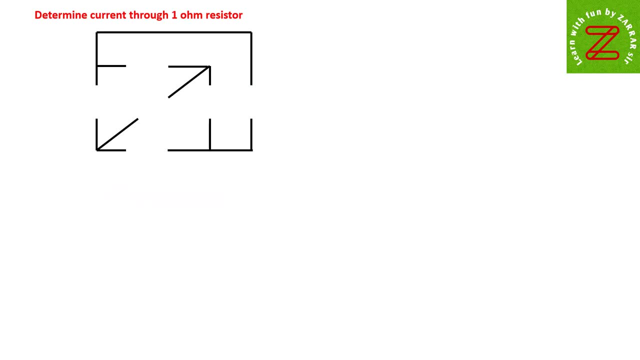 circuit will look like this, so you can see the current source has been removed. okay, what is the value of resistance that we have considered over here? the value of resistance over here was 3 ohm. okay, the value of resistance over here was 2 ohm. here also, I have considered 2 ohm. 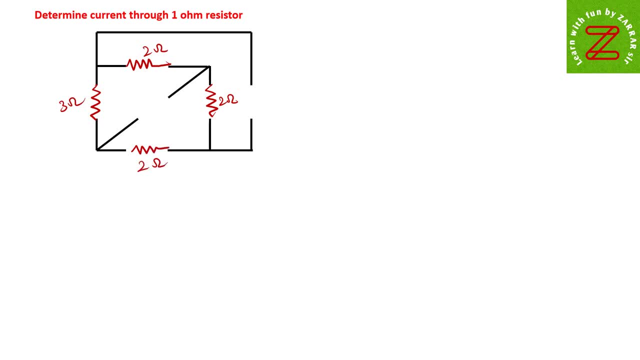 and here also it was 3 ohm, so I thought that I should add the voltage source here: 2 ohm, and this is what our important resistor, the value of this resistor, was 1 ohm. okay, and the final is voltage source, and you are aware about the voltage sources. the voltage, 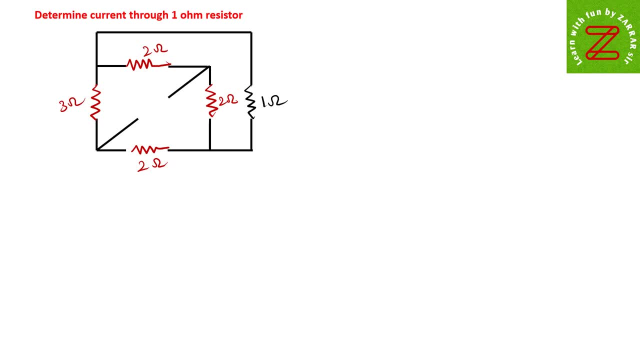 source. what we have considered is 4 volt, sorry, sorry, 1 volt. so this is the important voltage source that we need to consider, which is 1 volt. okay, i'm very sorry, let's write it properly: this is 1 volt. okay, now let's apply. so now move to step 2. i'll write step 2. 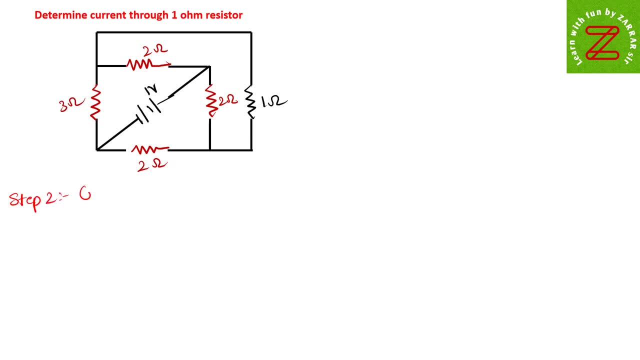 considering, i'll consider 1 volt source acting alone. if i'll consider 1 volt source acting alone, i'll apply kvl in this 2 loop. okay, if i'll apply this kvl in 3 loop, i'll now name it as i1, i2 and i3. okay, and you are now being 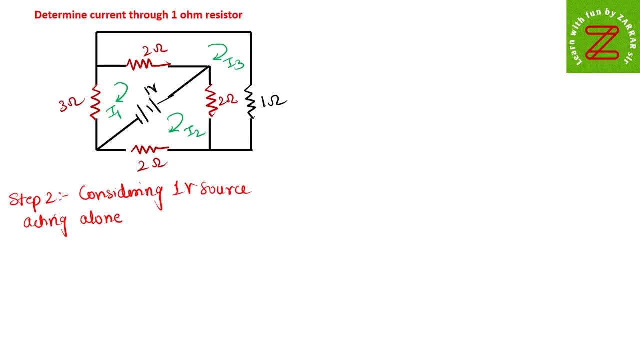 very perfect in applying kvl. let's apply kvl. i'll apply kvl in loop 1. if you apply kvl in loop 1, what will happen? try to understand the equation: if you apply kvl in loop 1, you will get 3. 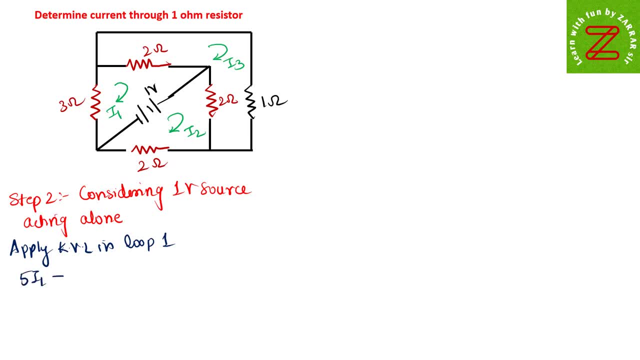 plus 2s, 5 i1 minus. this 2 ohm is in third loop also. so 2 i3 is equal to. you are moving from. as you can see, you are moving from positive to negative. you need to subtract, so you'll write minus 1. so this is your equation number first. now, similarly, i'll apply kvl in loop 2. now, if i. 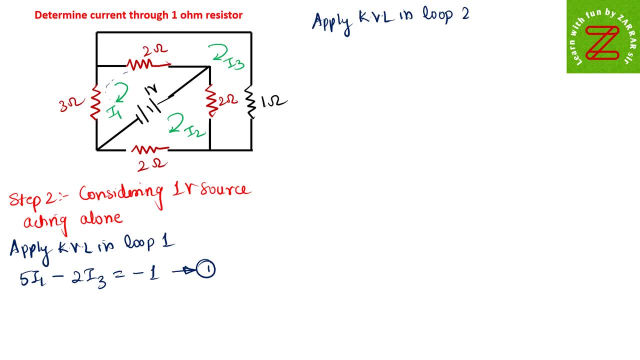 apply kvl in loop 2. 2 plus 2 is 4. okay, and i'll apply kvl in loop 2 and i'll apply kvl in loop 2. 2 plus 2 is 4 minus this 2 ohm is in i3 also, so 4 i2 minus 2 i3 is equal to: and now you are moving. 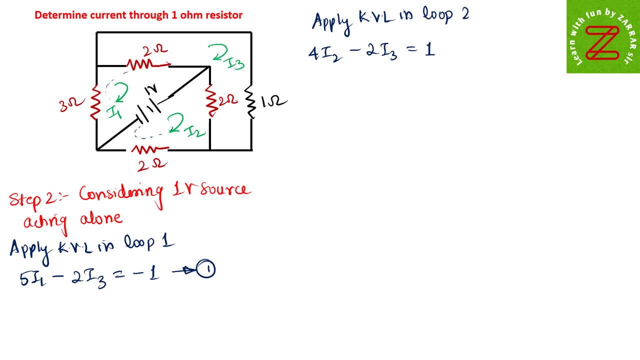 from negative to positive. that means you'll write positive plus 1. so this is my equation number 2. okay, so very simple. now, if i apply kvl in loop 3 and you can see if i apply kvl in loop 3, this is my loop 3. add all the resistance of loop 3: 2 plus 2 is 4, 4 plus 1 is 5, so it is 5 i3 minus. 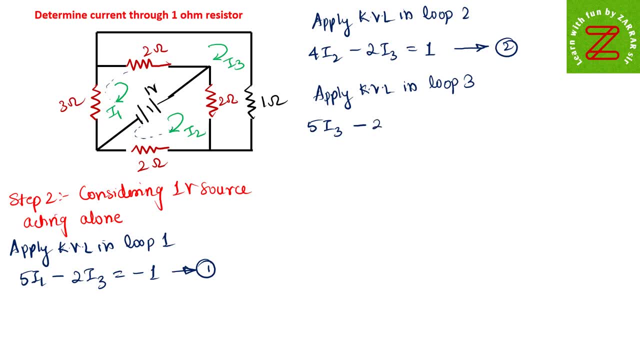 2 ohm is in first loop, so minus 2 i1. 2 ohm is in second loop and the current are opposite in direction, so minus 2 i2 is equal to. there is no voltage source in the third loop is equal to 0. 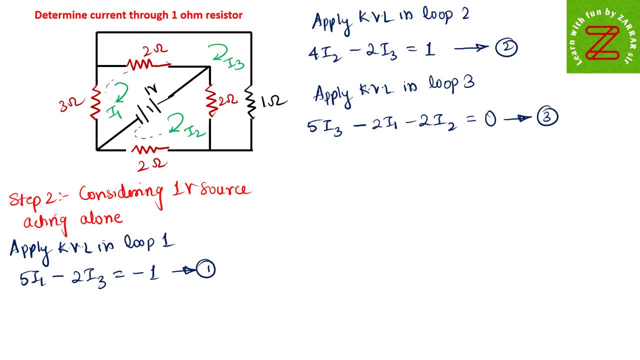 so this is my third equation. hope you have understand all the three equations. now, once you have got all the three equation, you'll use the calculator to solve all this simultaneously and you'll get the value of i1, i2 and i3, and i've already solved it for you. 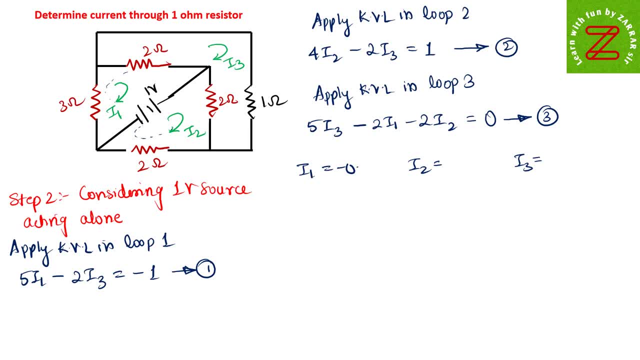 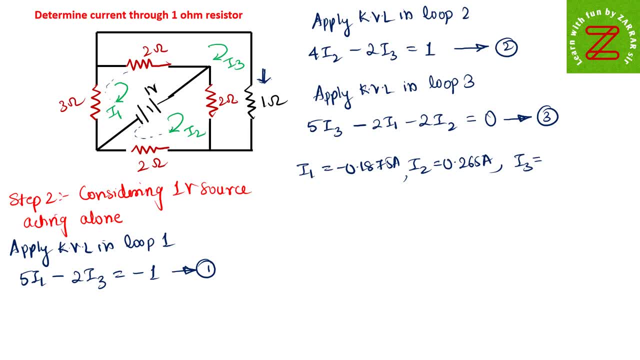 loop because i 1 ohm is in third loop, so i3 is directly. you can write i3 as 0.031, 0.031 ampere. okay, and i double dash will be i3, which is equal to 0.031 ampere. 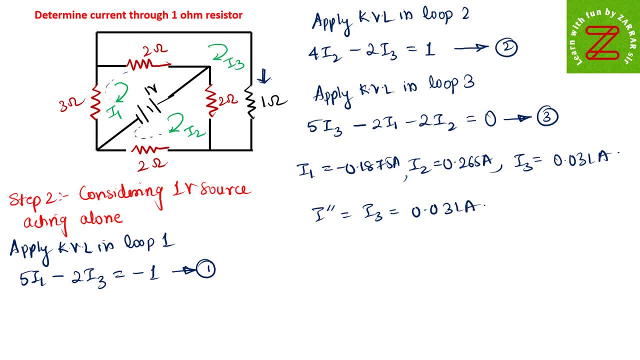 so now my total using superposition theorem. if i use using superposition theorem, using superposition theorem, i will be i dash plus i double dash, which is equal to 0.375, which we have already got, plus 0.031 ampere, and this is finally equal to 0.406 ampere. hope you have. 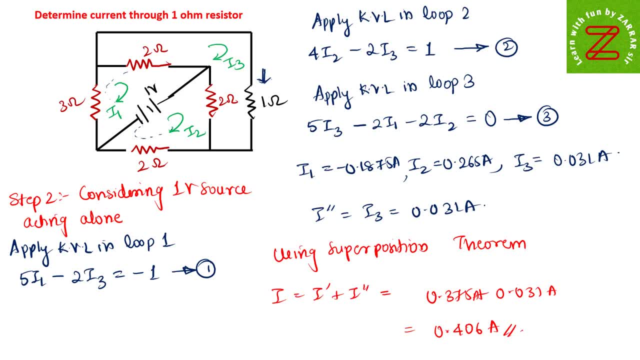 understand superposition theorem. this was the superposition theorem, please, uh, this is the final answer. please like the video? subscribe my channel and comment if you understand this, so that i can upload thevenian and norton in the next video. thank you, guys. have a good day.